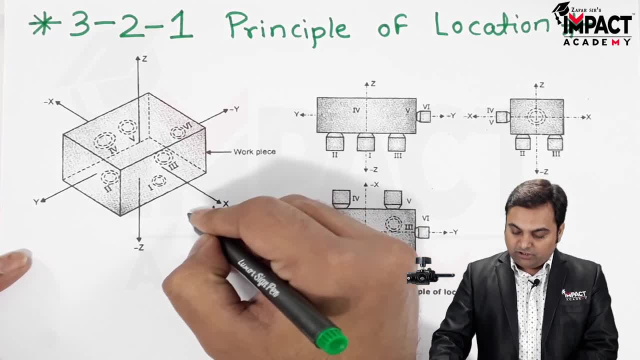 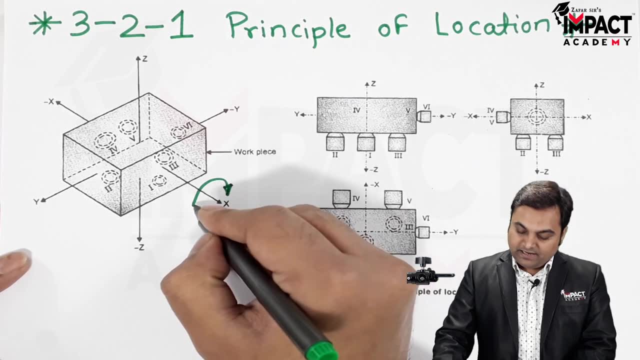 After that, the same object can move. It can rotate along x direction, in the clockwise direction, when I'm looking along the positive x. At the same time it can rotate in an anti-clockwise sense as well, along the same direction. 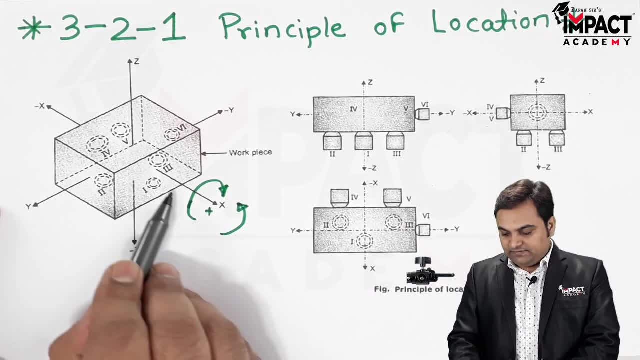 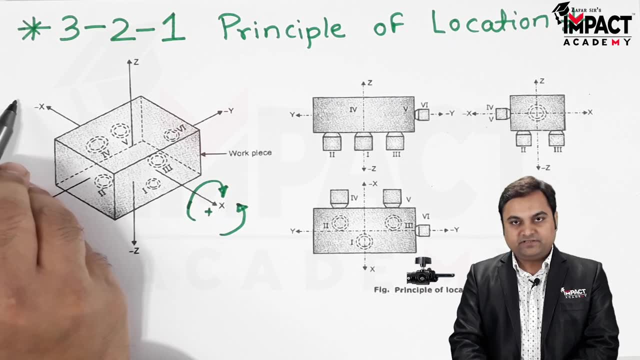 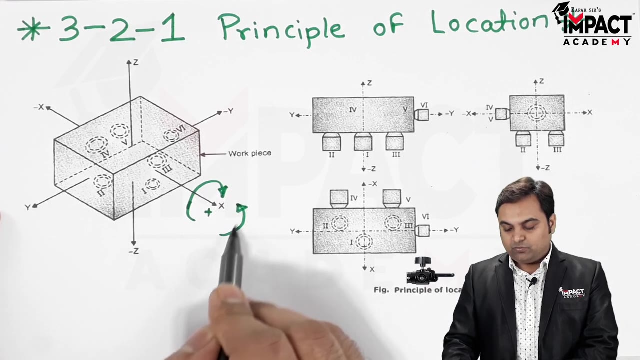 So here we can say that translation along x, that is positive x, 1 degree of freedom. Translation along negative x, that is 2 degree of freedom. Clockwise rotation about x, That is 3 degree of freedom, And anti-clockwise rotation about x, that is 4 degrees of freedom. 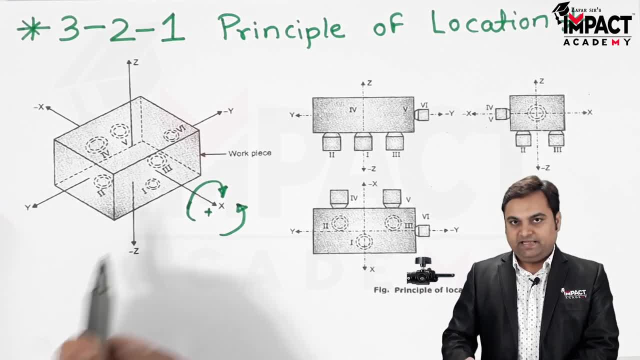 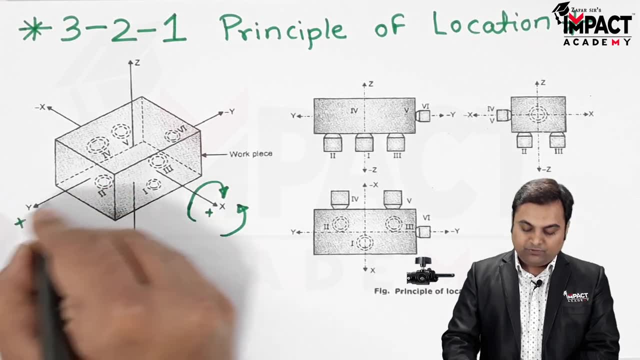 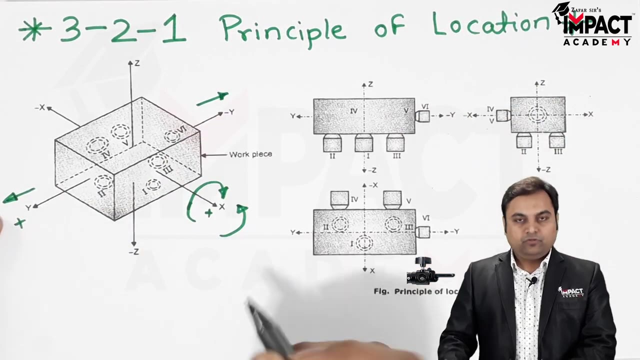 So 4 degrees of freedom are there along the x direction or x axis. Similarly, when we go for the y direction, we have translation along positive y, translation along negative y, So both the translations, so they become 2 degree of freedom. 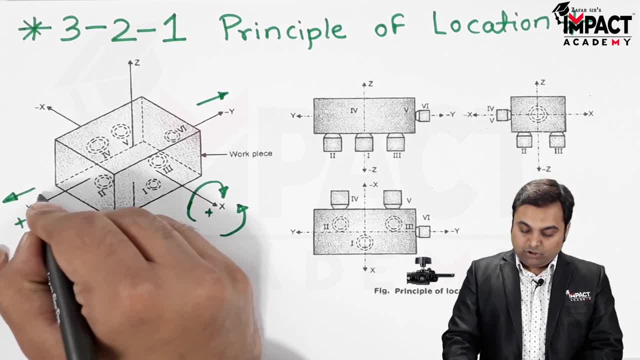 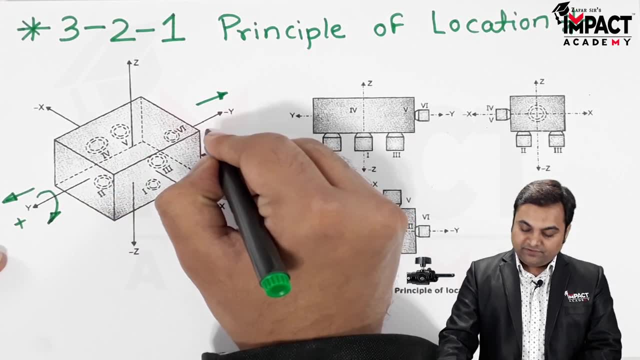 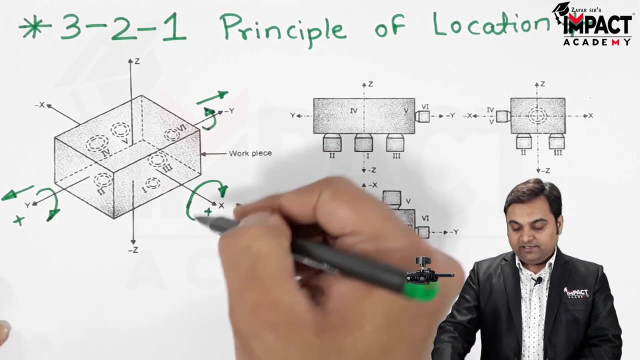 Similarly, while looking from the positive y direction, Object can rotate in a clockwise manner, Then it can also rotate in an anti-clockwise sense. So again we have 4 degrees of freedom along y. Similarly, like we had in x, like in x, we had translation along positive x, along negative x. 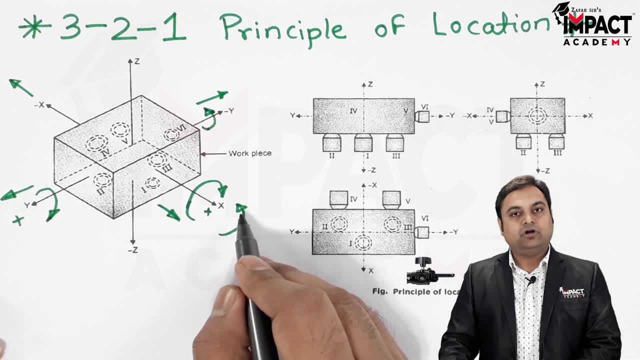 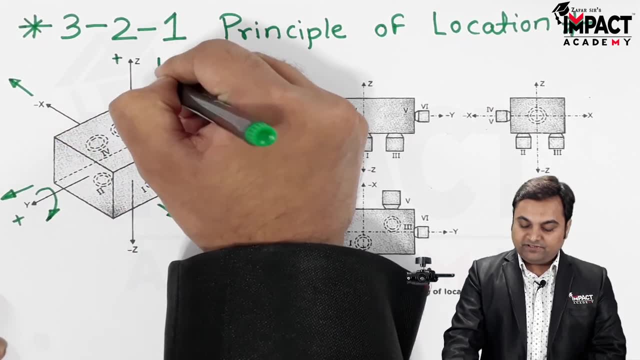 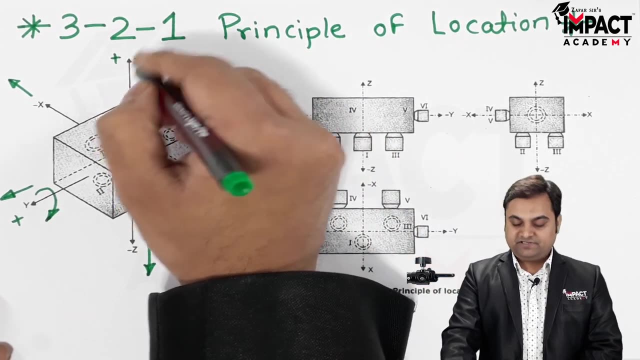 And at the same time rotation of clock and anti-clock along x direction, Similarly for y, And the same thing goes for z direction as well. So along the positive z there is translation, Translation, along negative z, And at the same time, when I am looking from positive x direction, there is clockwise rotation. 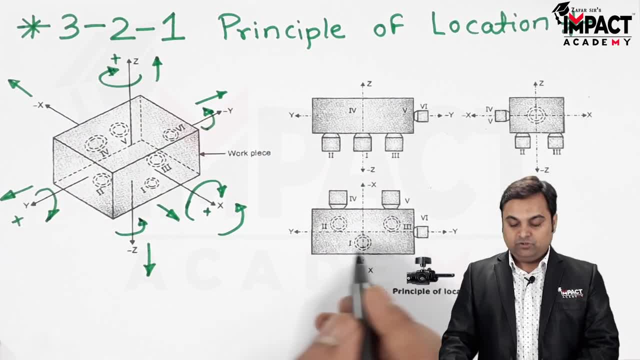 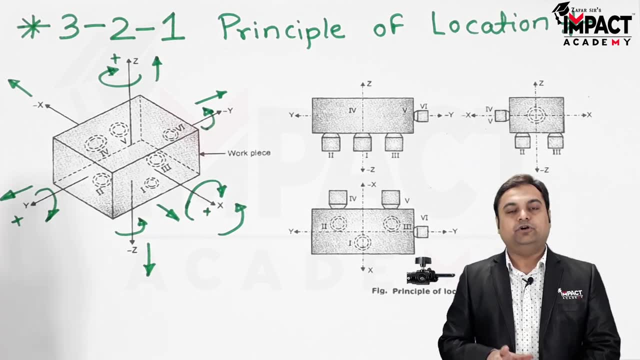 And at the same time there is an anti-clockwise rotation. So we can say that when we add up all these degrees of freedom, the value comes out to be 12.. It means a free body which is kept in space has 12 degrees of freedom. 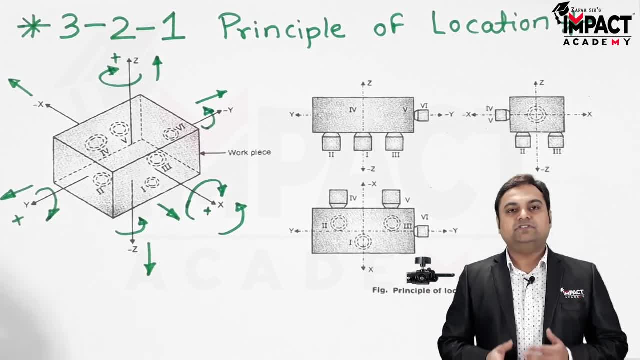 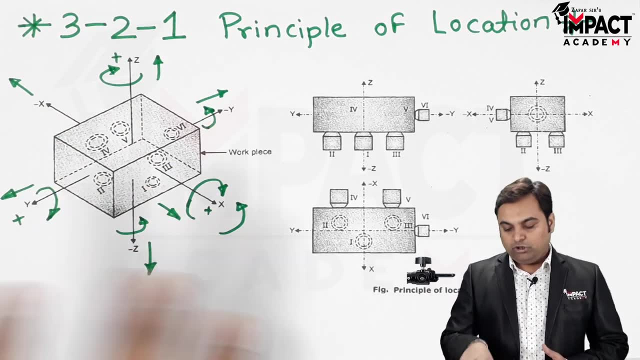 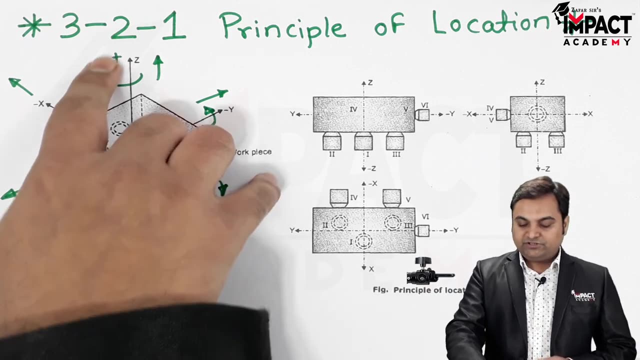 Now this body can be considered as the work piece on which we have to perform the machining operation. So we have to restrict these degrees of freedom. It means all the 12 degrees of freedom should be restricted. So in order to restrict these degrees of freedom, we are using the 3 to 1 principle of location. 3 to 1 means we have 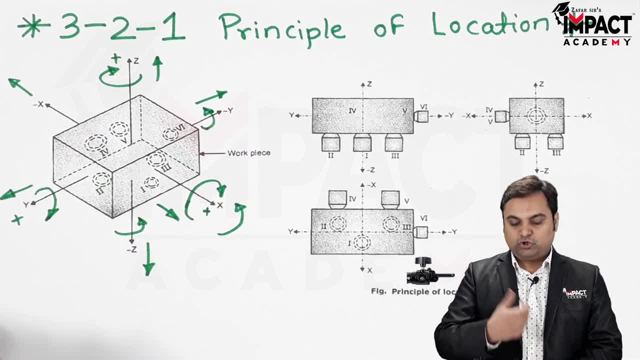 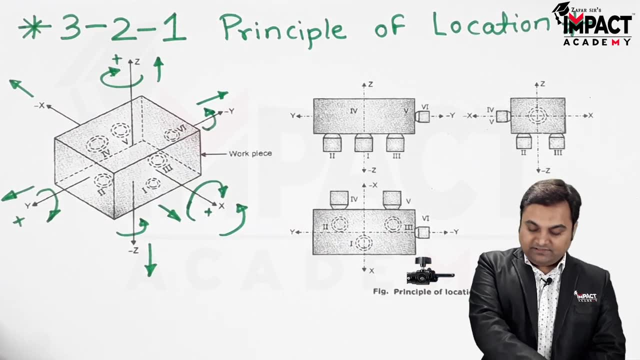 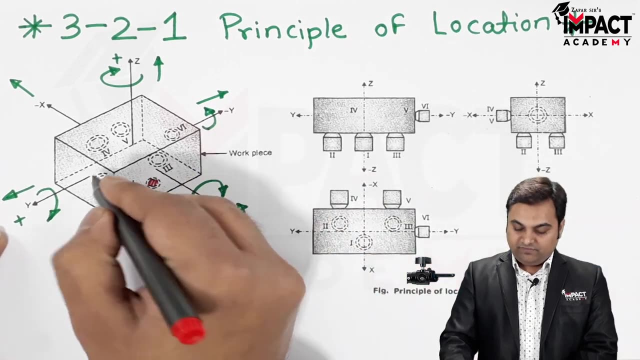 three pins, rest pins, also called as support pins or pad. So we have three pins, two pins and one, and the location method is like, for example, at the bottom, when we see here in the bottom plane there are three pins, That is, this is pin number one. here we have pin number second and pin third. 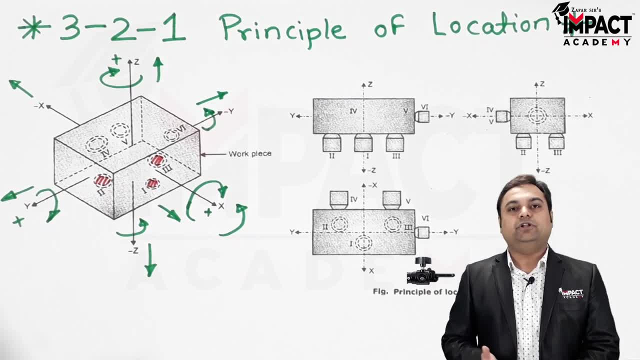 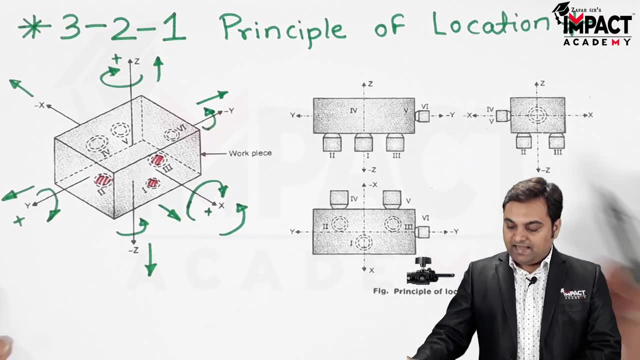 So these pins needs to be attached in the body of the jig or fixture on which this component is to be kept. So here we have three pins, and it is shown in this diagram as well. At the bottom plane we can see there are three pins. 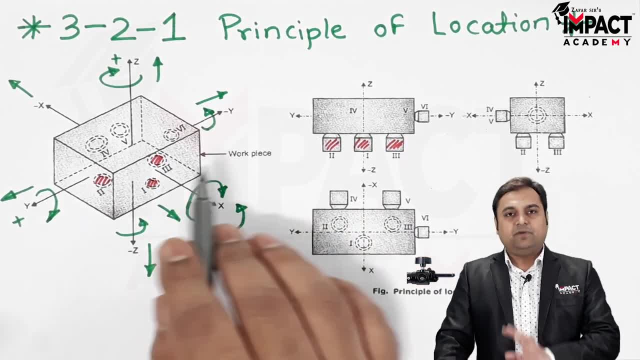 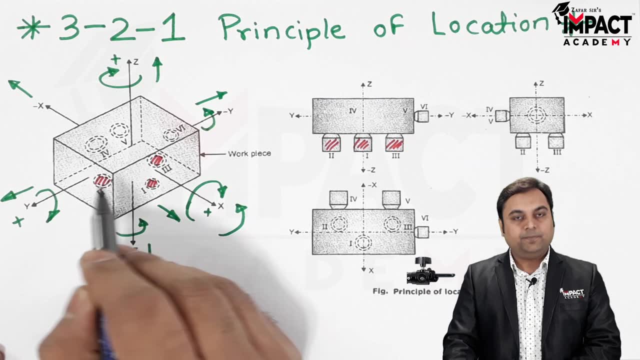 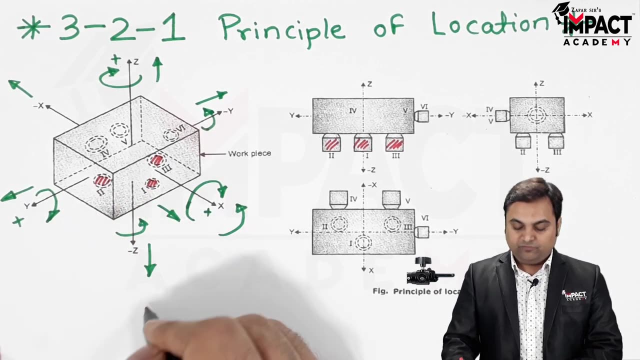 So now, with the help of these three pins, some amount of degrees of freedom would be restricted, and which are restricted. that I'll explain. First of all, with the help of all these three pins, the downward movement along z direction is. restricted, means now the object cannot move. 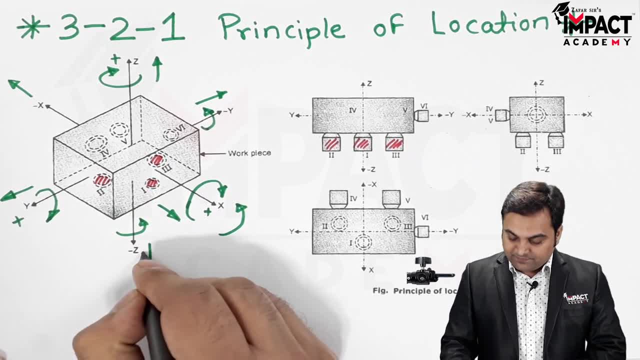 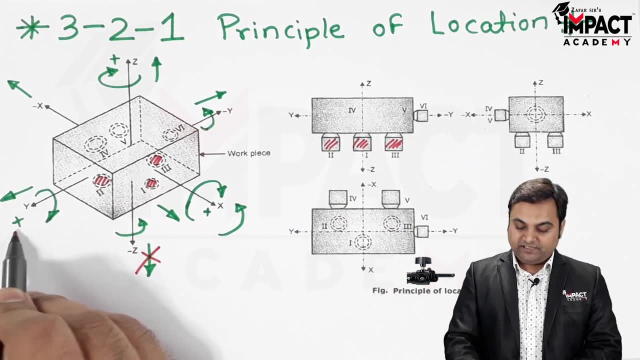 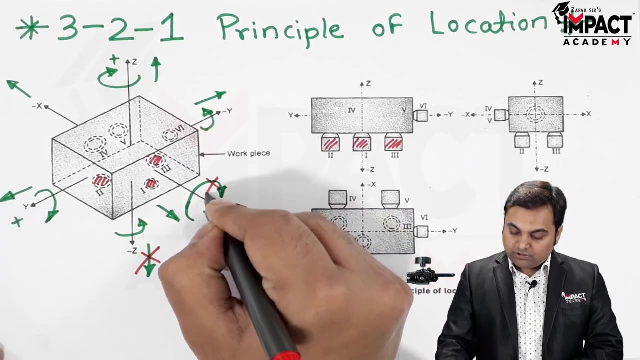 in the downward z direction. So this degree of freedom has been cancelled. Similarly the object now, when it is kept on these three pins, it cannot rotate along The x direction as well as the y direction. So rotation along x, both clock and anti clock. 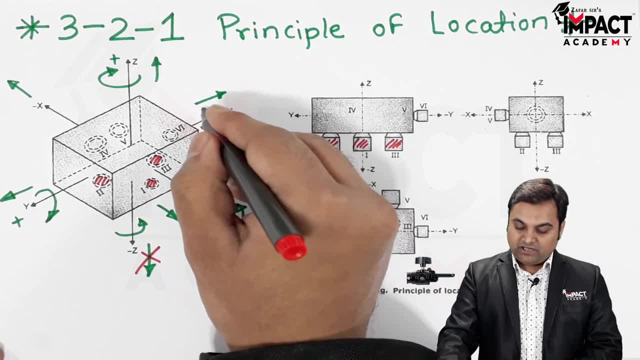 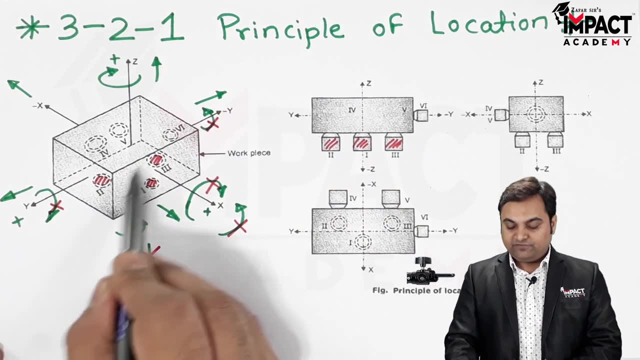 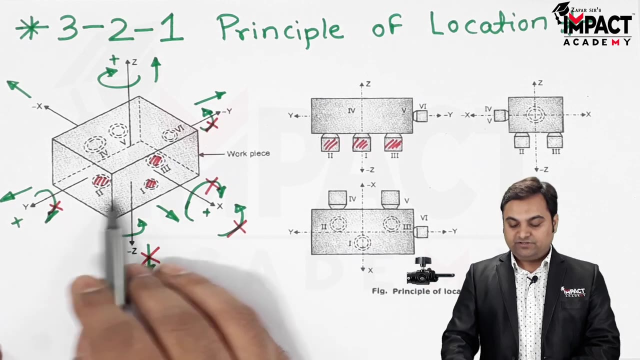 has been restricted. Similarly, the rotation along y clock, as well as anti clock, has been restricted. So just by the introduction of these three pins, the total degrees of freedom that are restricted are 1, 2,, 3,, 4 and 5.. So by using three pins, five degrees of freedom have been arrested. Now for the 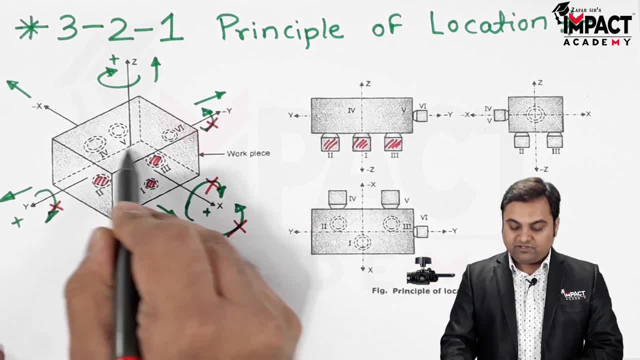 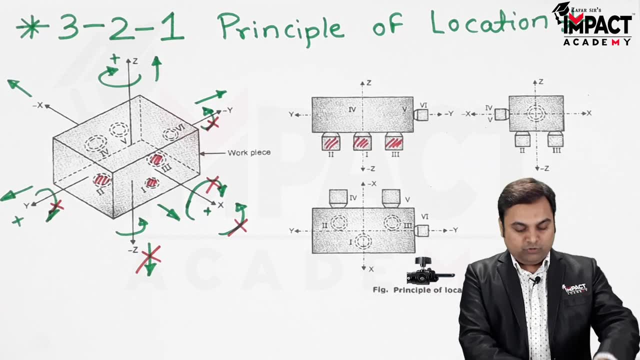 Here, perpendicular to this plane, where we were having 3 pins, that is, 1st, 2nd and 3rd, there is a plane over here In that we are introducing 2 more pins, that is, pin 4 and pin 5.. 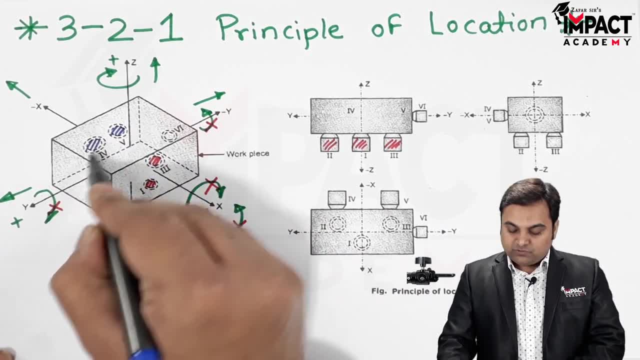 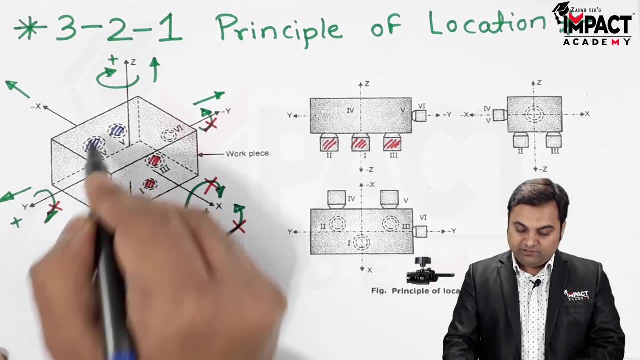 Now, when I am having these 2 pins, which are perpendicular to the plane of the pins carrying 1, 2 and 3.. Because of the introduction of these 2 pins, that is, 4 and 5, the movement along the negative x direction, that is, translation, is arrested. 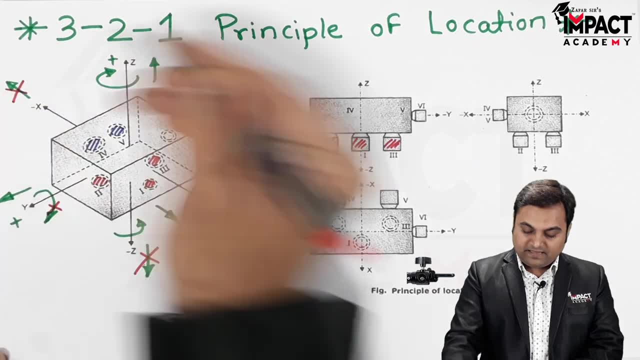 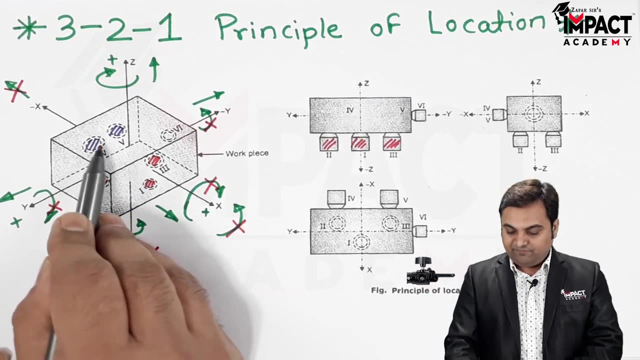 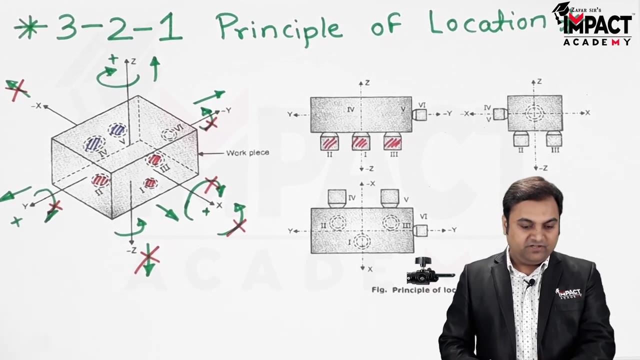 It means the degree of freedom is cancelled over here. So now we can see that by the introduction of 3 plus 2, that is 5 pins, we have restricted 6 degrees of freedom. Then at the same time we can say that now the object. 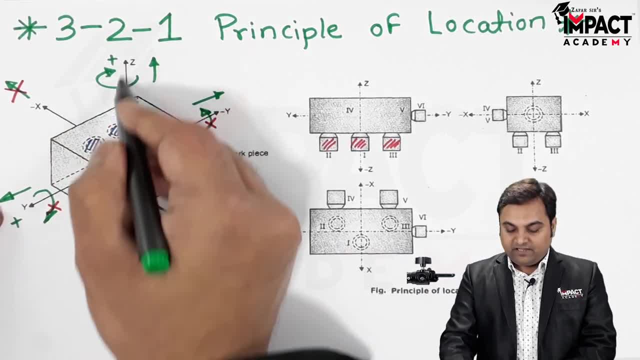 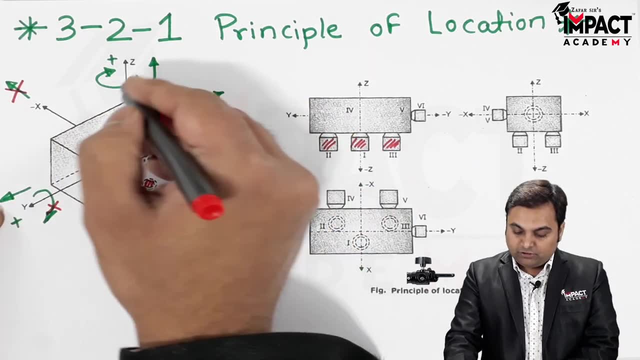 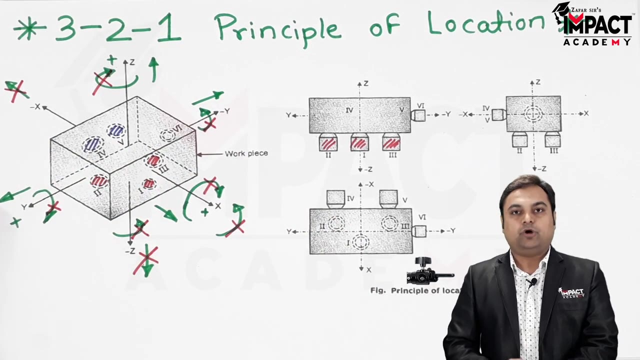 Also cannot rotate along the positive or we can say along the z direction. So by the introduction of pins 4 and 5, the object cannot rotate- in a clockwise sense and anticlockwise sense- along z direction. So the total degrees of freedom which are stopped or restricted now becomes 8.. 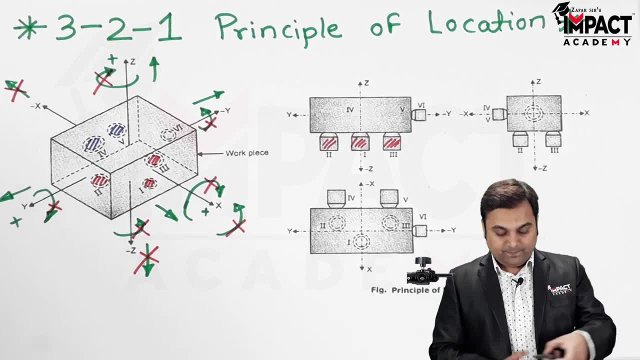 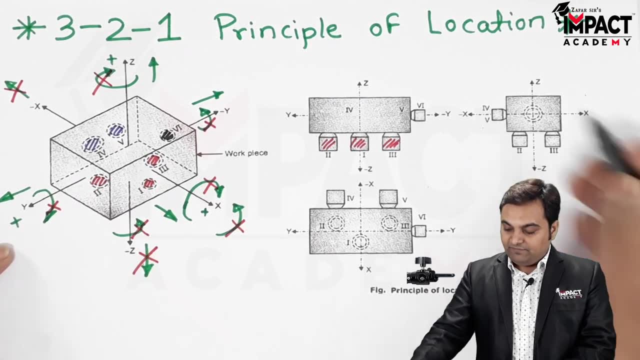 After that, we are going to introduce another pin along the plane which is perpendicular to both these planes carrying 1, 2, 3 and 4, 5. That is pin 6.. And we can see it over this diagram as well. 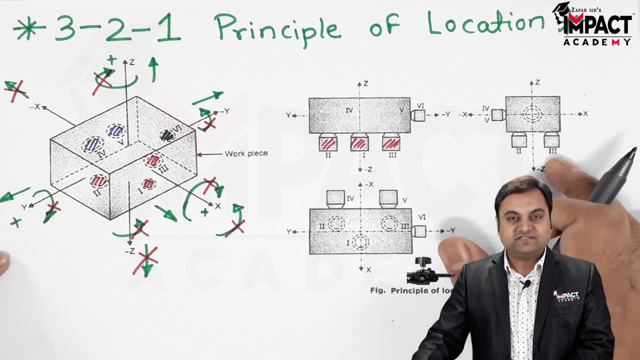 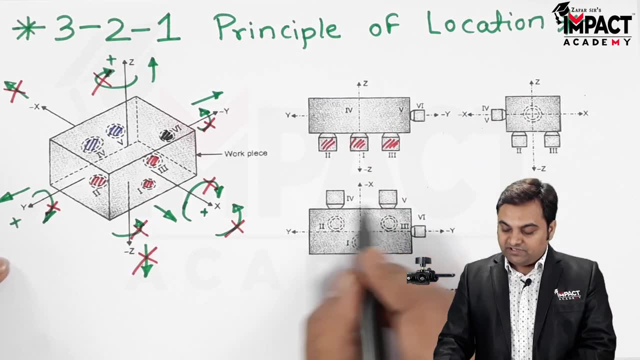 That this is the front view. here we have top view and this is the side view. So in the front view there are 3 pins, that is, 1st, 2nd and 3rd. Opposite to that, when we see here in the top view, we have pins 4 and 5.. 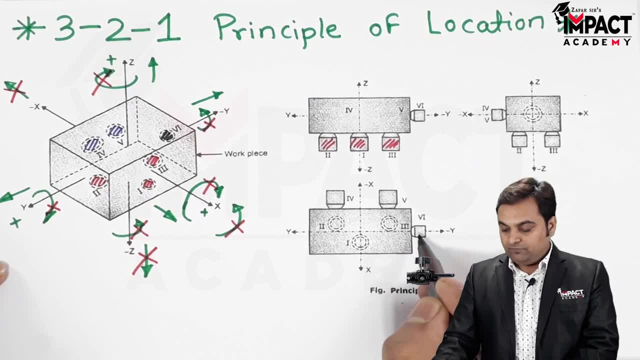 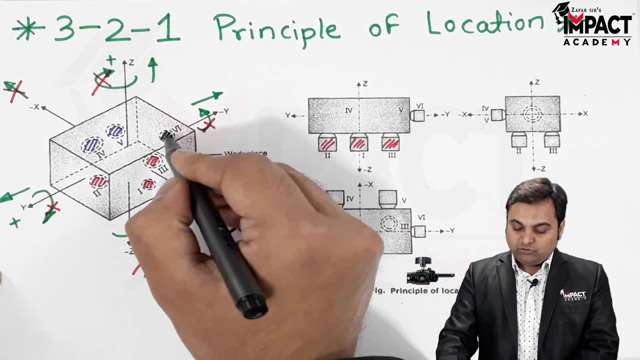 And perpendicular to both these planes we have another plane on which there is pin 6. we can see it over here. So just by the introduction of this pin, which is pin 6, now the object cannot move in the negative y direction. So that degree of freedom has been restricted. 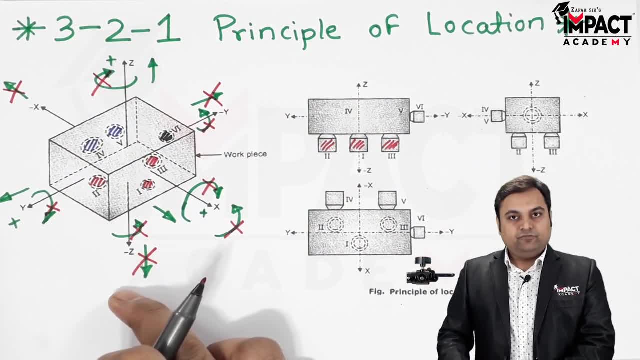 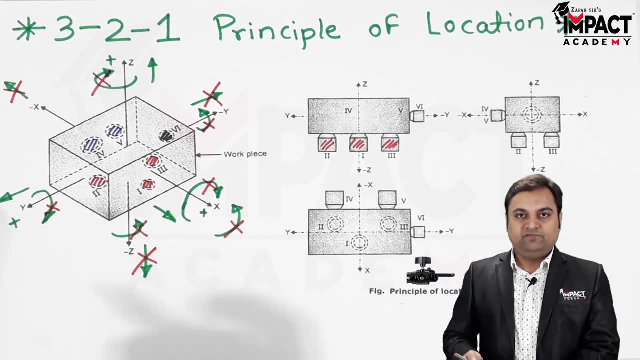 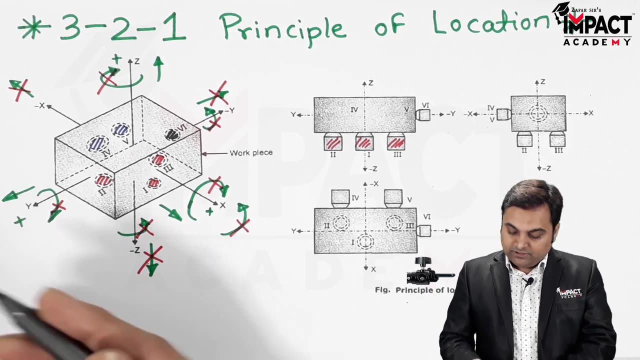 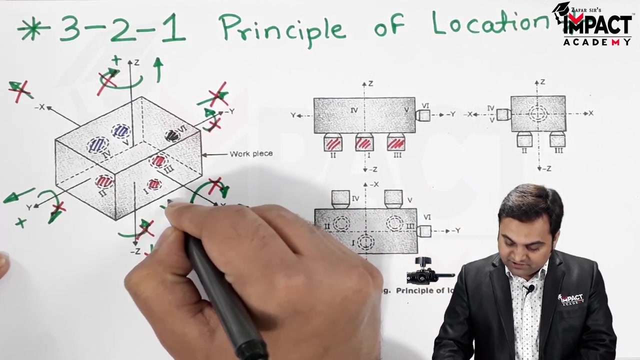 So when we add up all the values, we are getting that 9 degrees of freedom have been arrested just by using 6 pins. So out of 12, 9 degrees of freedom has been restricted. Now whatever remains here we can see that still we can say there can be positive movement along the x direction means positive translation is there? 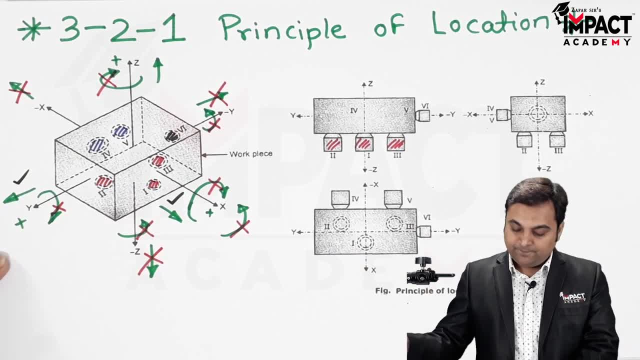 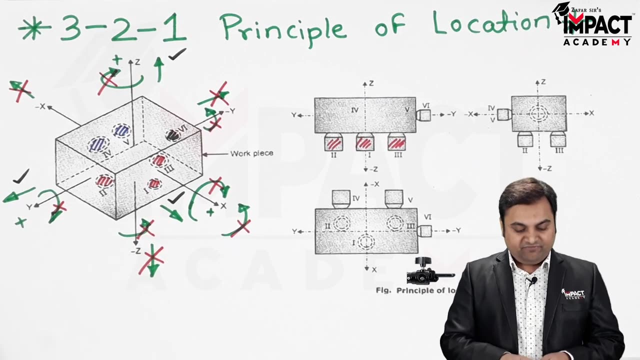 Then positive translation along y is there and positive translation along z is there. It means out of 12,, 9 degrees of freedom have been restricted, but still 3 degrees of freedom are there. So we cannot add. if we are going to add more number of pins over here, then what may happen is it becomes difficult to load and unload the work piece. 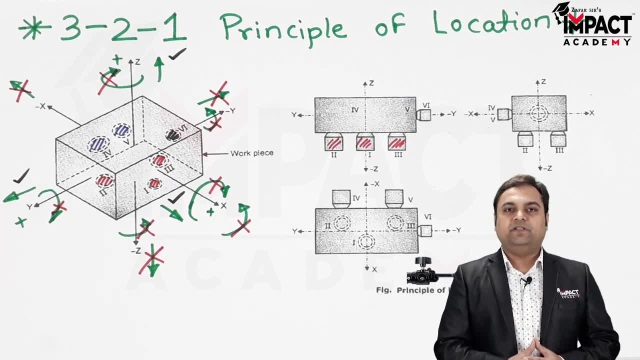 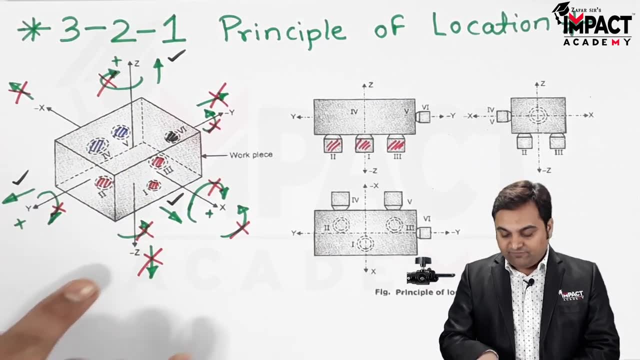 So the concept is such that we have to use minimum number of pins And stop maximum degrees of freedom. So by using 6 pins, 9 degrees of freedom has been restricted and for these remaining 3 degrees of freedom. that is translation along positive x. the object can move.